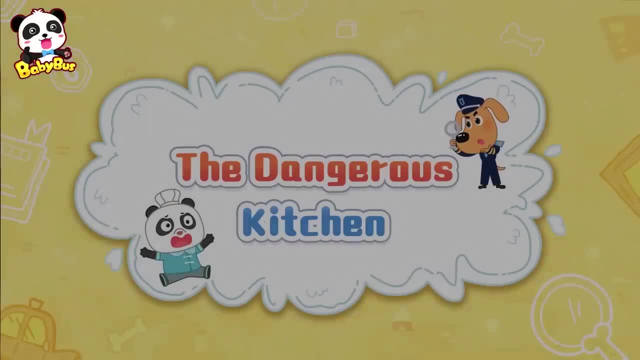 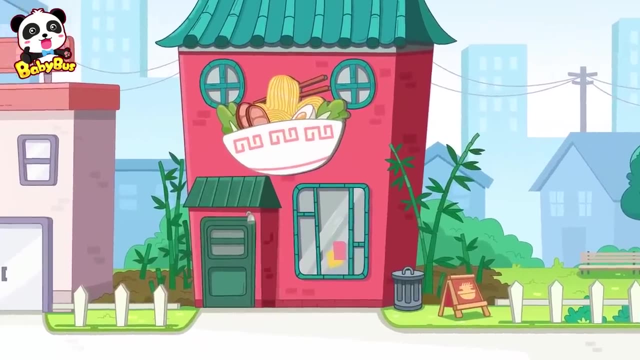 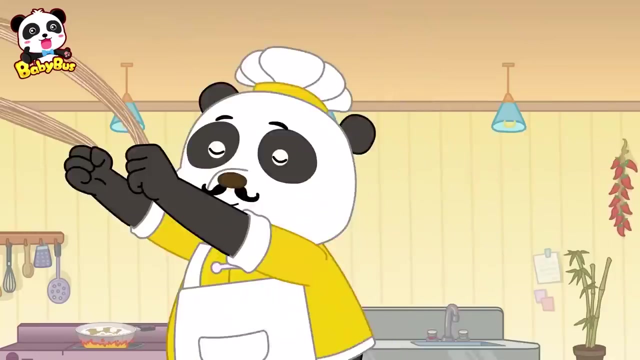 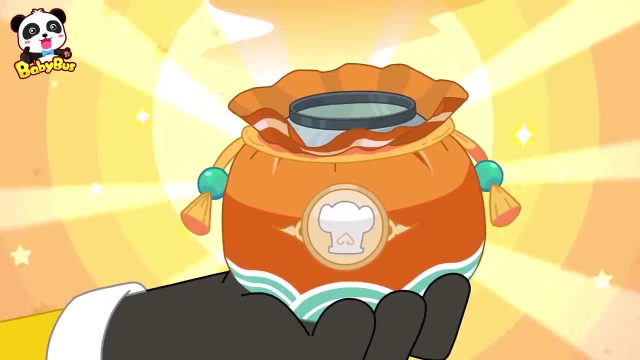 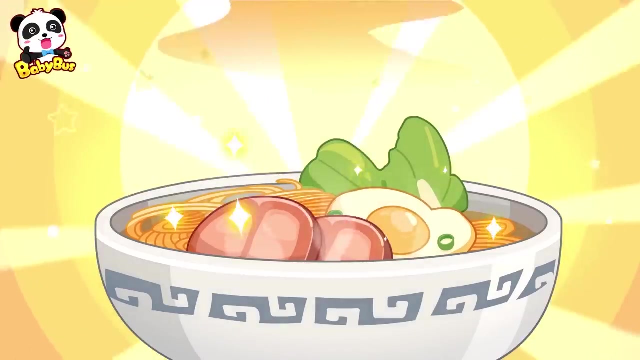 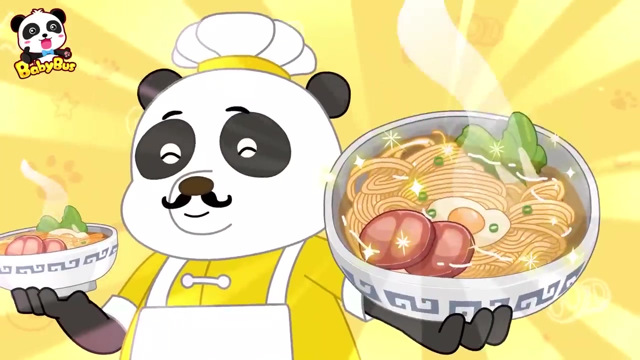 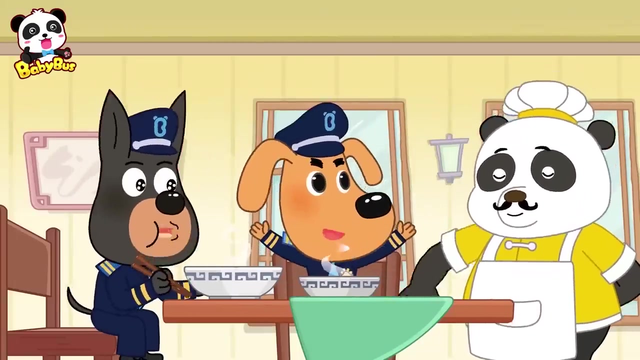 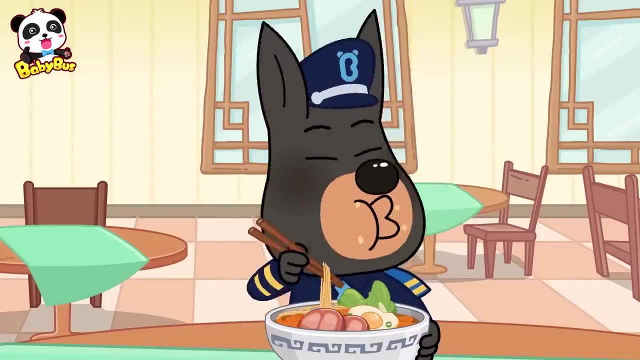 Baby Bus. The Dangerous Kitchen Smells so good. Two bowls of our signature noodles- Wow, It looks so yummy. Mr Panda, your noodles are amazing. That's because of our secret spice mix. Secret spice mix- Yeah, The recipe's from our daddy's, daddy's daddy. 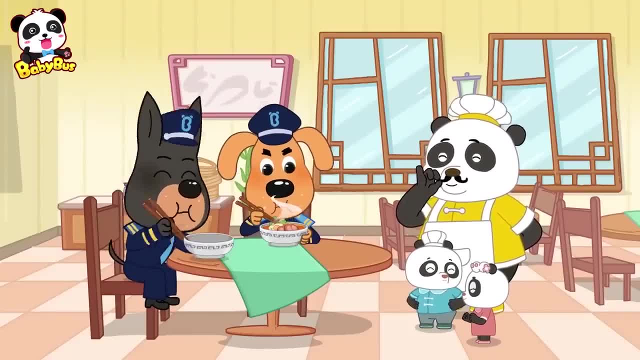 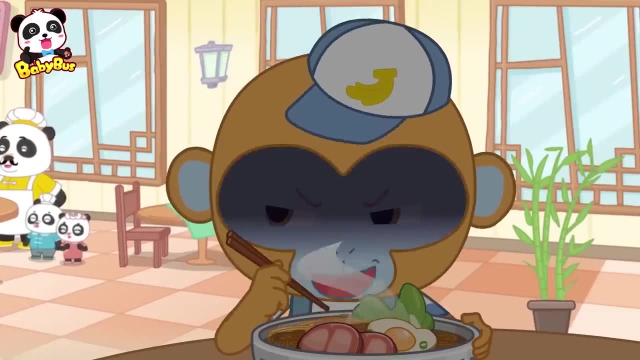 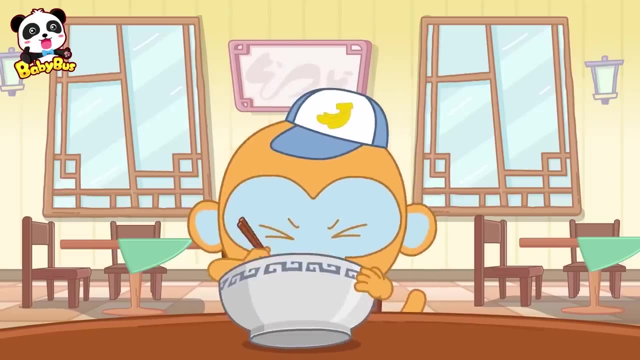 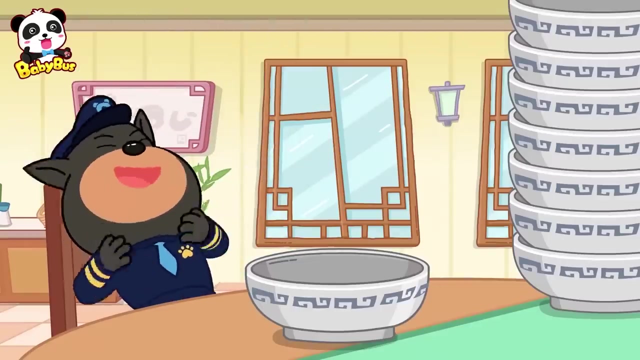 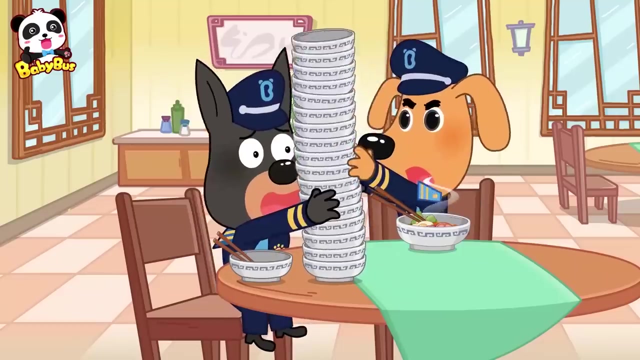 That's right. Another bowl please. If I had the secret spice mix, I'd be able to make yummy noodles too. Amazing. Another bowl please, Mr Panda, My spice mix. What happened? Let's go and have a look. 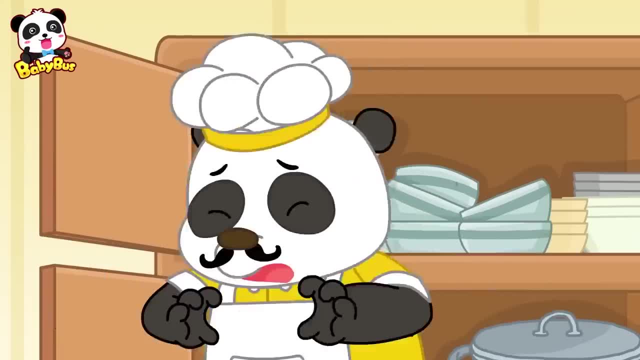 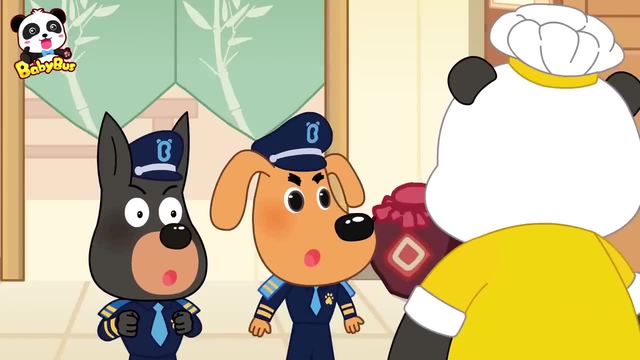 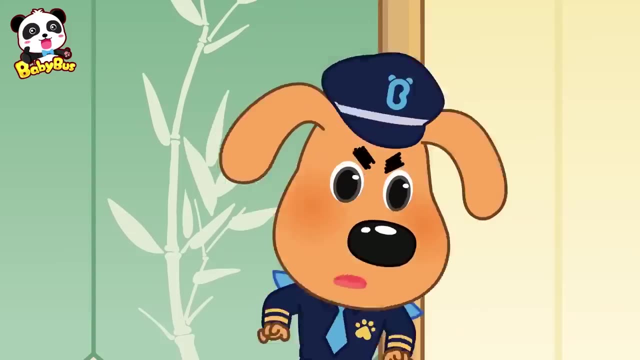 Mr Panda, what's wrong? Sheriff Labrador, my secret spice mix is gone. What It's handed down to me by my family and now it's gone. Please help me find it. Oh, Don't worry, There's no case that I can't solve. 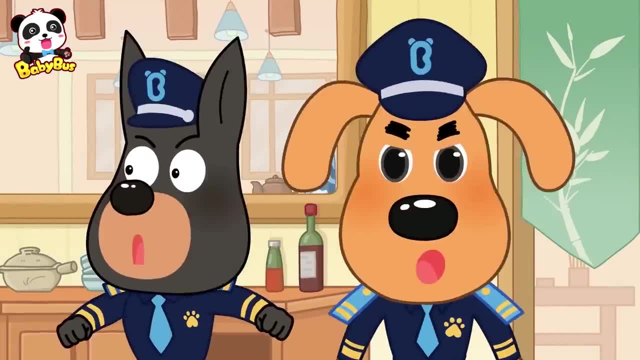 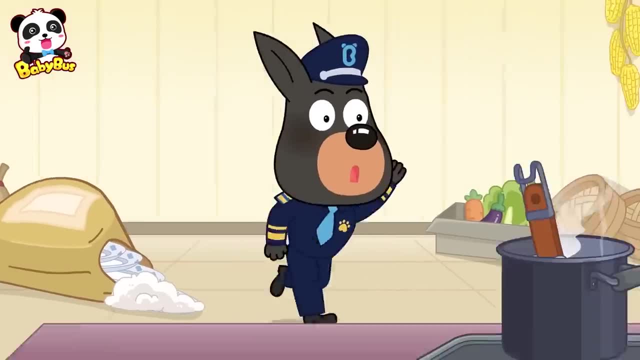 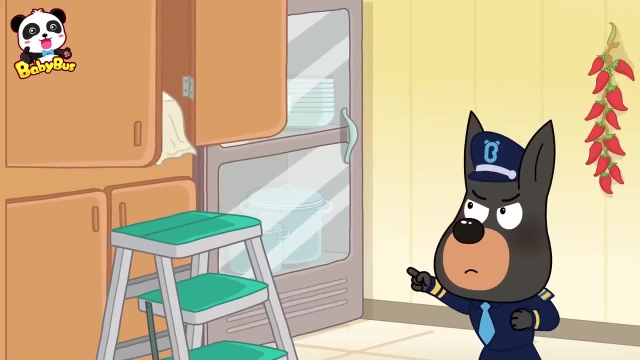 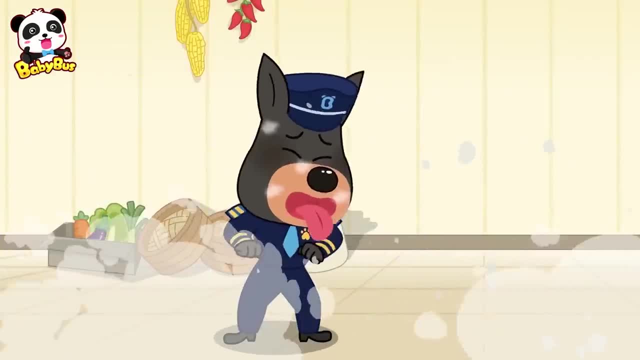 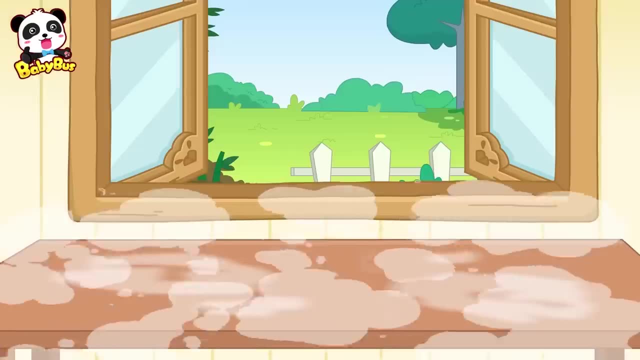 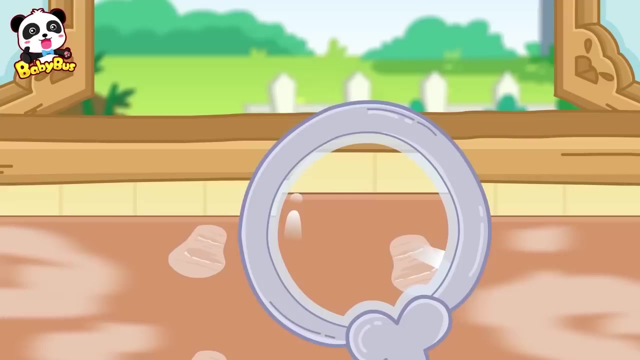 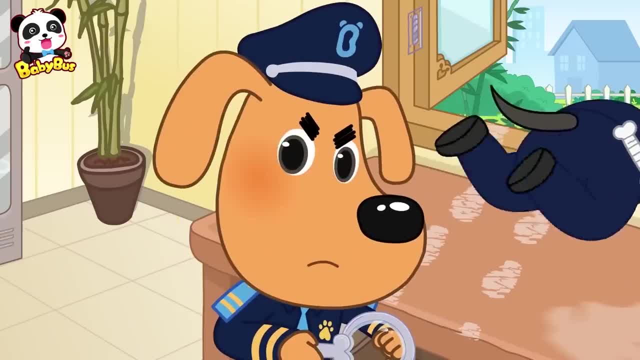 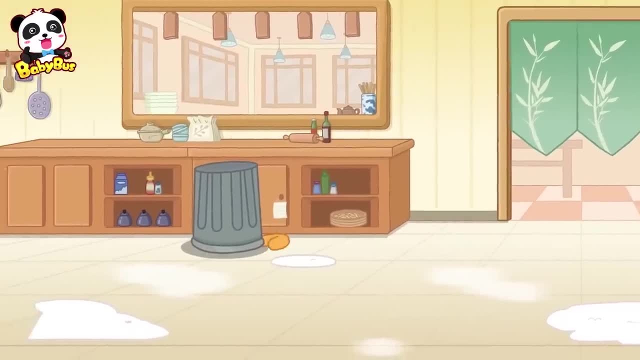 Wait, The thief might still be here. What Look? there are no footprints leading out of here, So the thief must still be here. Huh, You can't run away, I got you Ouch. Stop right there. 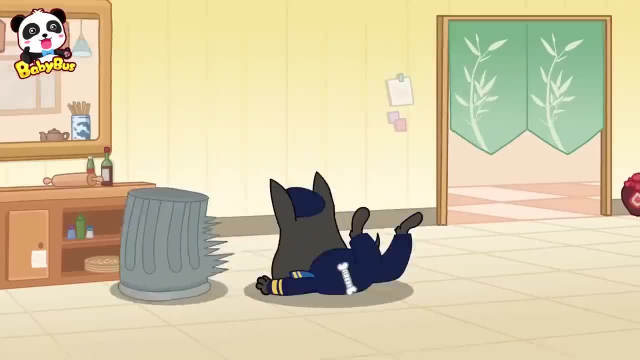 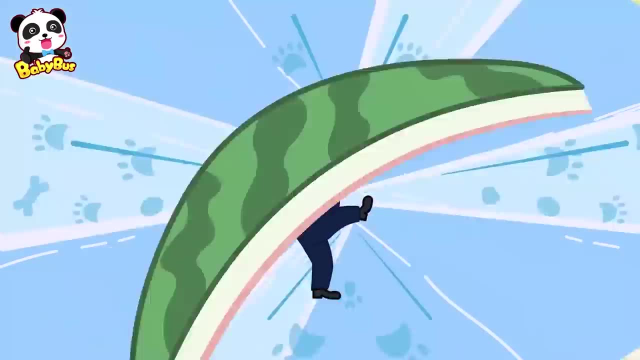 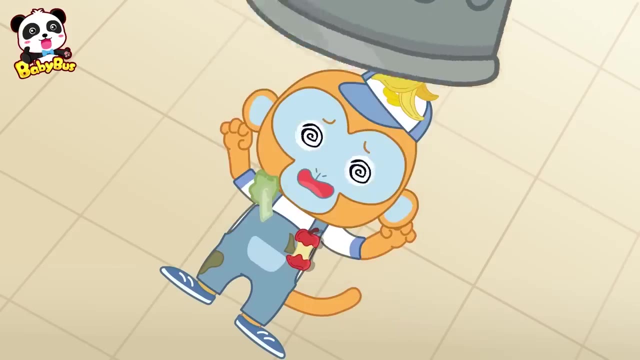 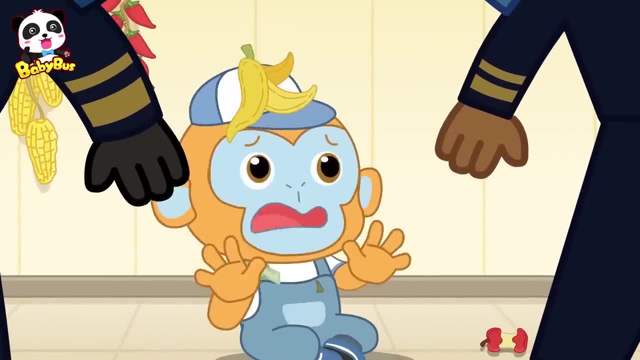 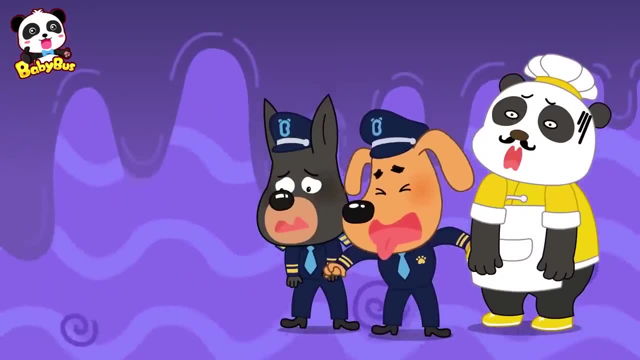 No, It wasn't me, I'm sorry. I just wanted to see how the noodles are made. I didn't steal your spice mix. You can search me if you want. Ah, Ah, Ah, Ah, Ah, Ah Ah. 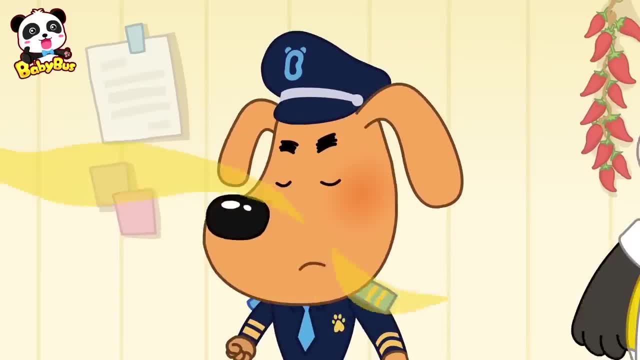 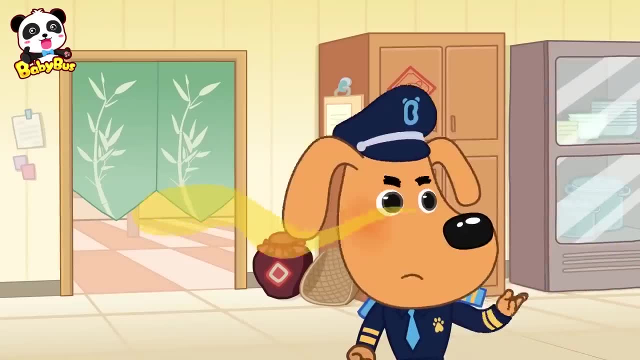 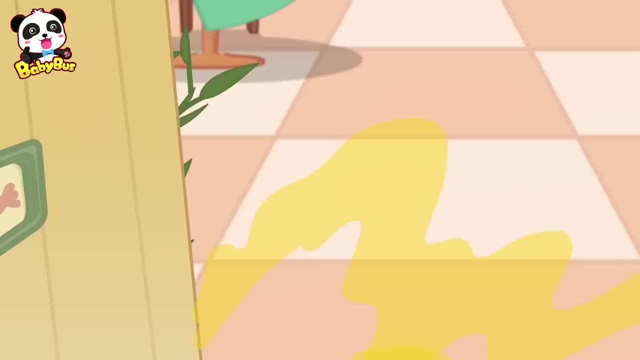 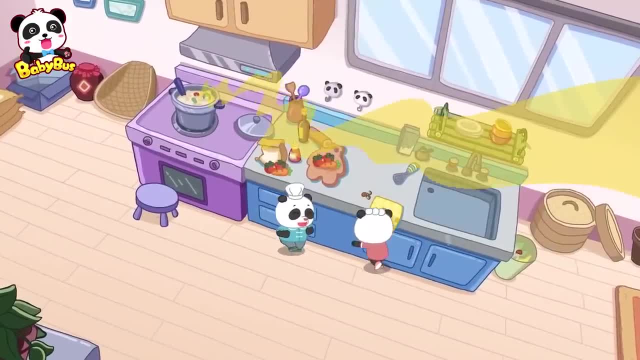 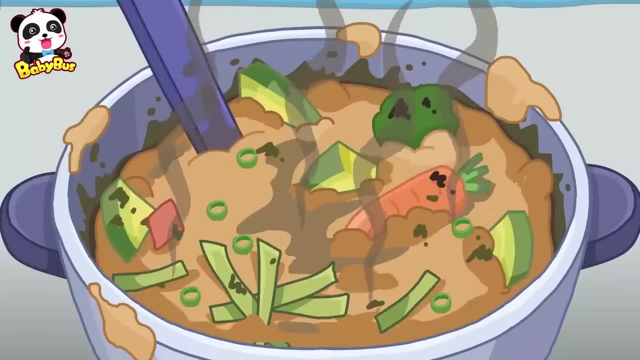 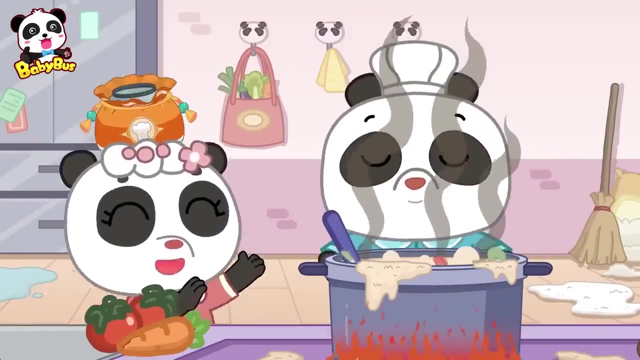 Come on, Let's go. Uh, Uh Uh. Tomato, Carrot, Mushroom, Cucumber. Hahaha, I'm the best chef in the world. Wow, Mr Chef, That's so cute. The secret spice Here. 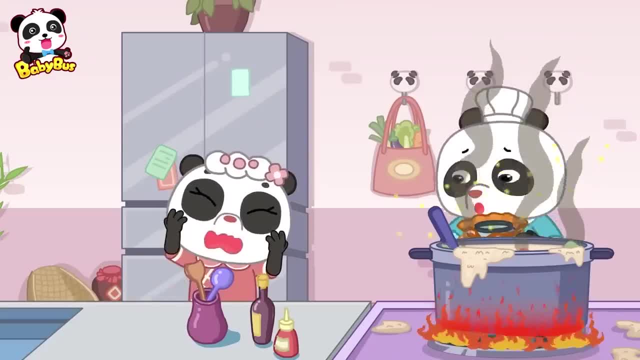 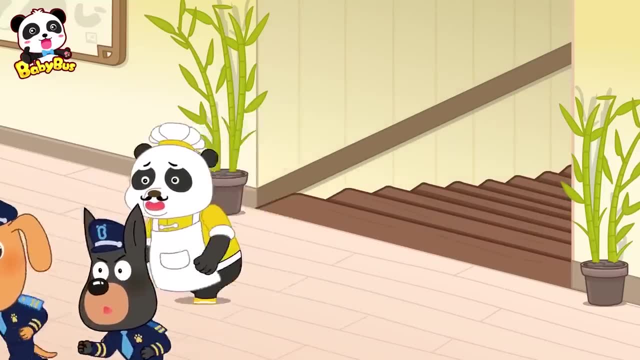 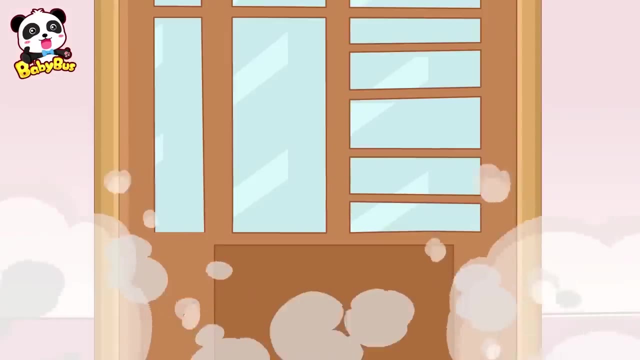 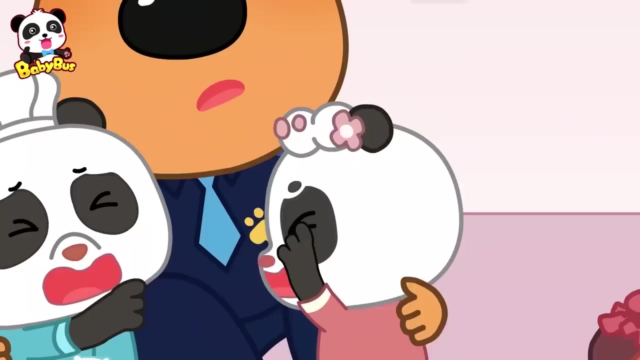 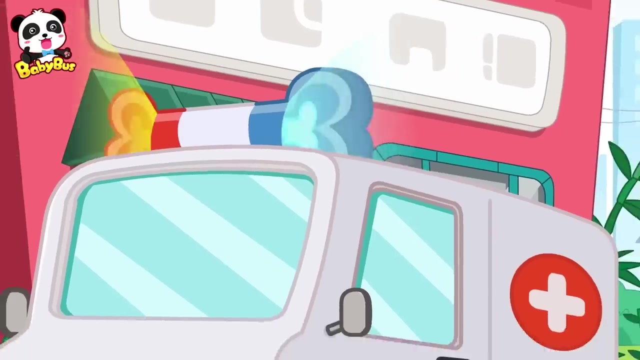 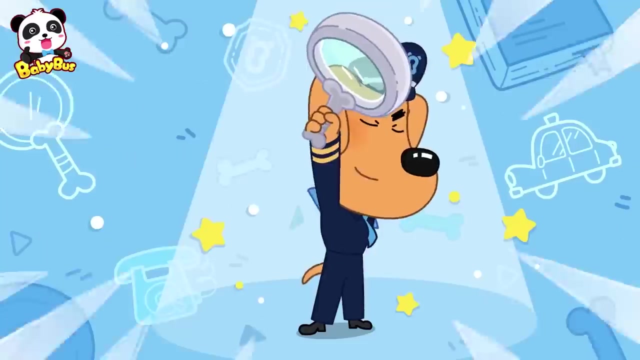 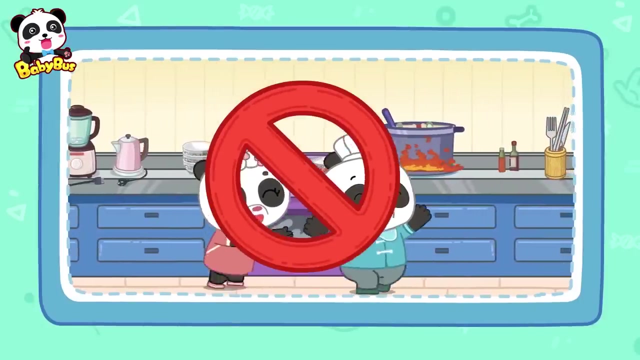 Wow, Ow, My eyes. It's my daughter. Hurry, Watch out, Let's go, My eyes. We need to send her to the hospital right now. Sheriff Labrador's Safety Talk. Kids never play in the kitchen. There are sharp knives and tools. 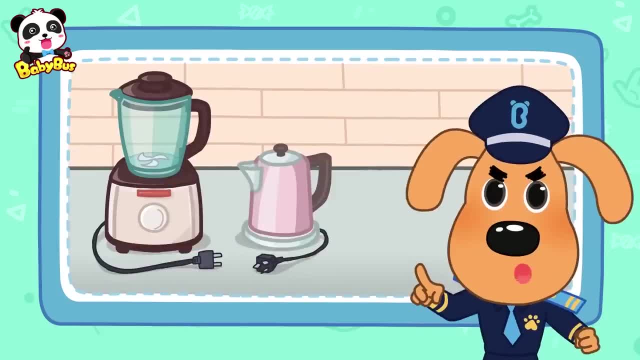 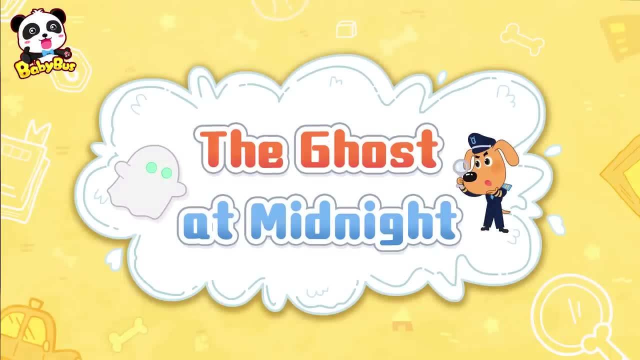 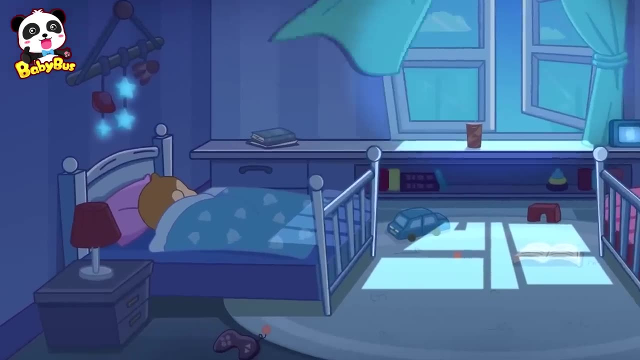 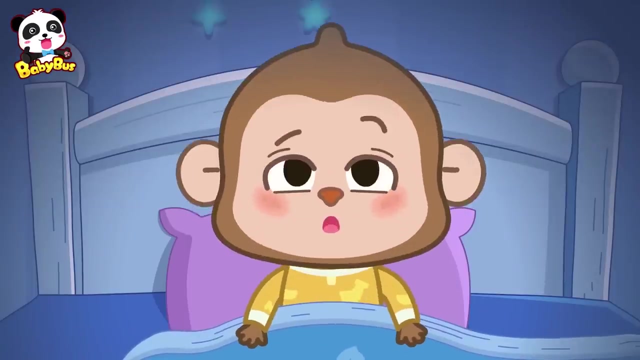 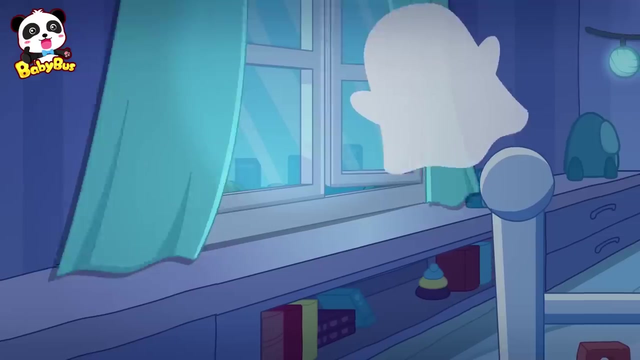 boiling water and electric appliances in the kitchen, And they can hurt you Also. parents need to keep an eye on their children when they're in the kitchen too. The Ghost at Midnight, Mommy, Mommy, Oh, what's wrong. 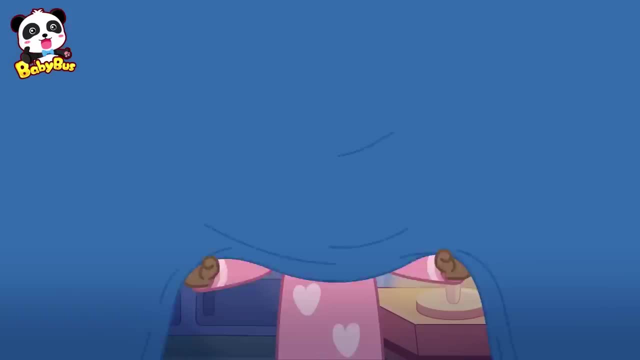 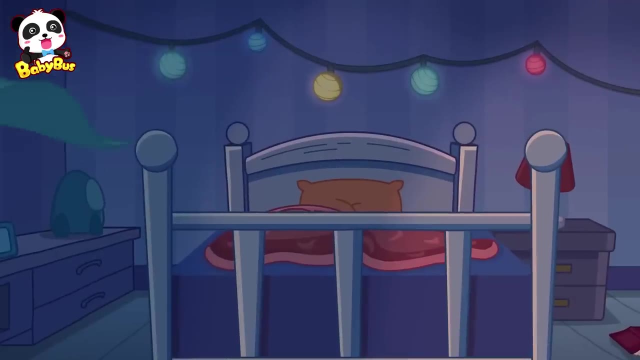 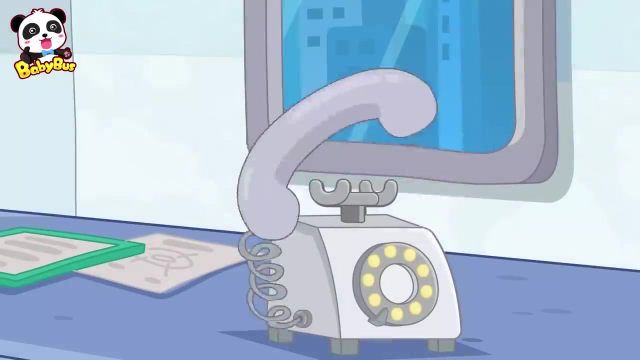 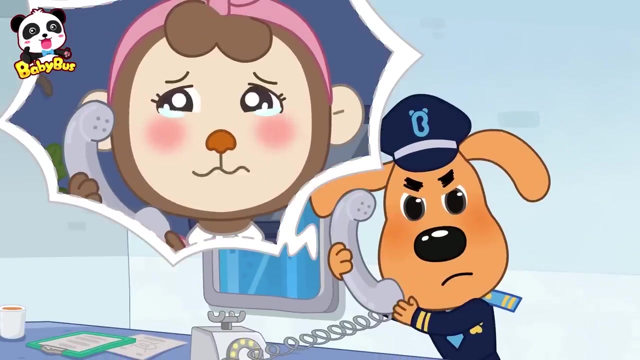 I saw a ghost. Don't be afraid, sweetie Mommy's here. Where's your sister? A ghost must have taken her. A ghost, Woof. Hi, I'm Sheriff Labrador. my daughter is missing. Please help me find her. 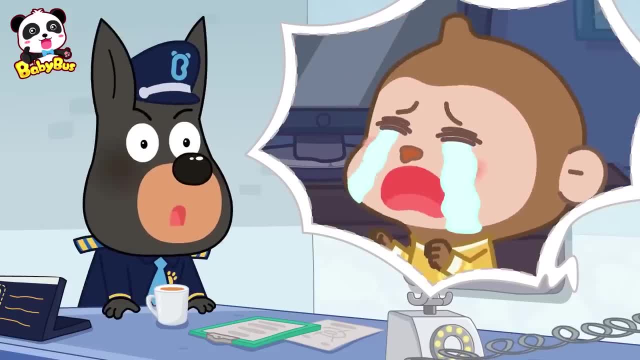 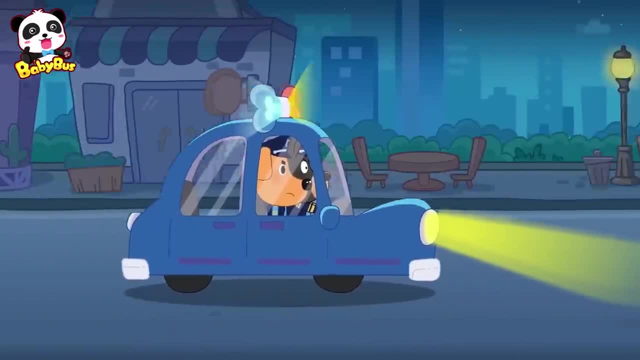 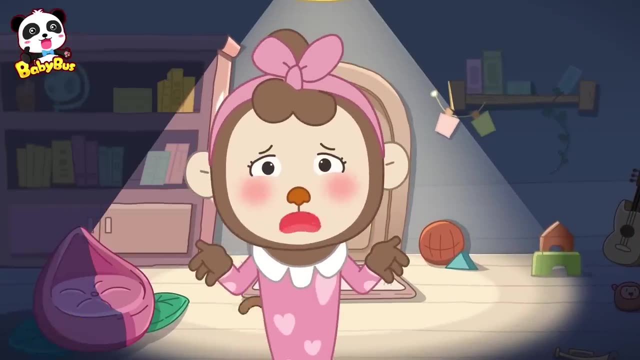 A ghost took her. A ghost, Don't worry, we'll be right there. Huh, Sheriff Labrador, my daughter was sleeping in this room and suddenly she disappeared. The ghost must have taken her. Hey, kid, there's no such thing as a ghost. 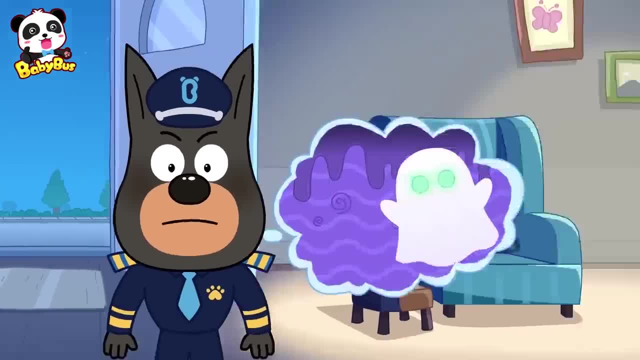 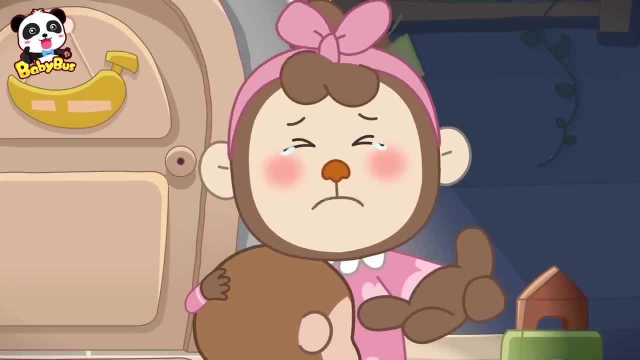 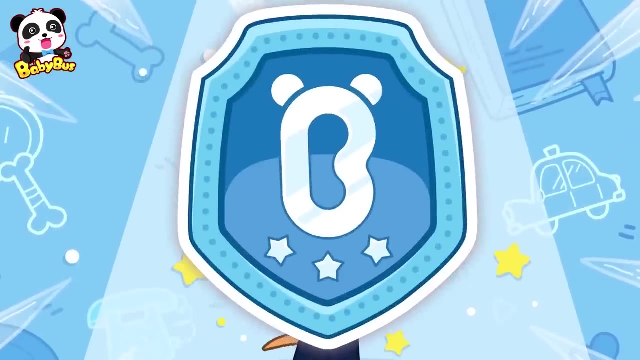 But I saw it. It was white and its eyes were bright and green. It was so scary. Oh Sheriff Labrador, please save my daughter. Don't worry, there's no case that I can't solve. Let's search Sister Monkey's room first. 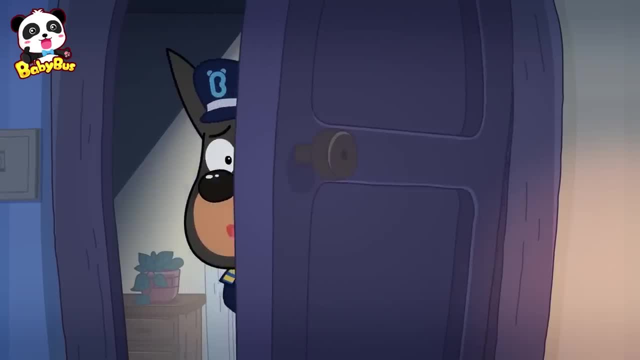 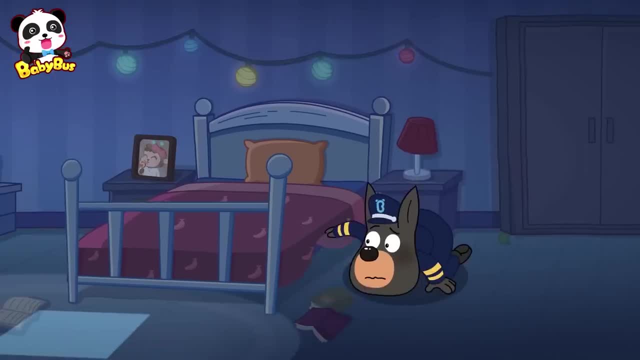 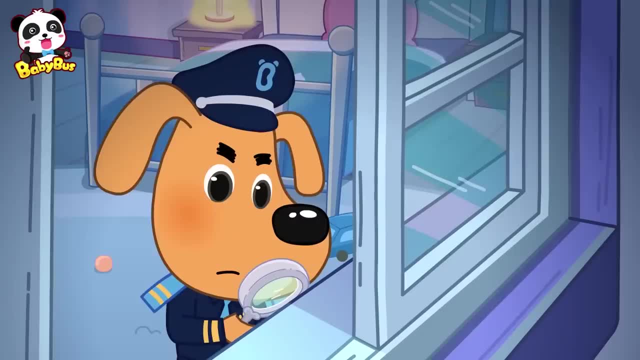 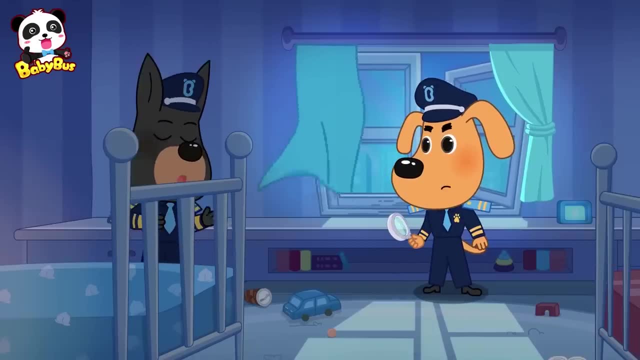 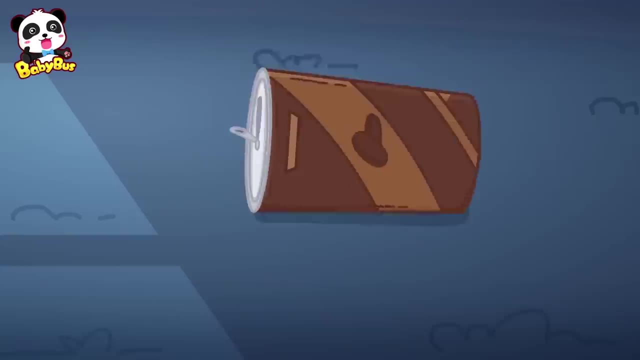 There are only child's footprints on the windowsill and there's no sign that the window was forced open. I don't think she was taken by anyone, So there is no ghost. Oh, Oh, Hmm, Hmm, it's coffee. 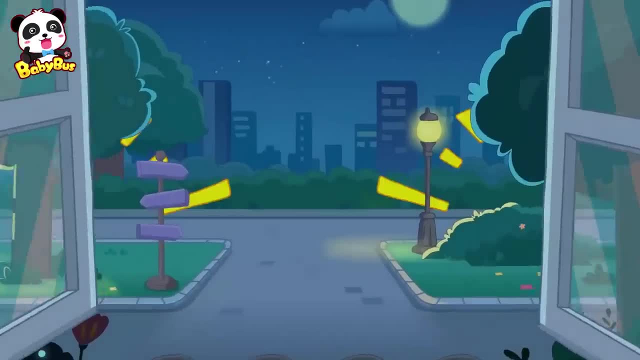 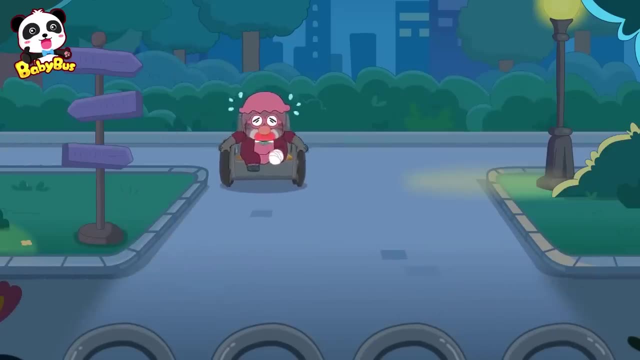 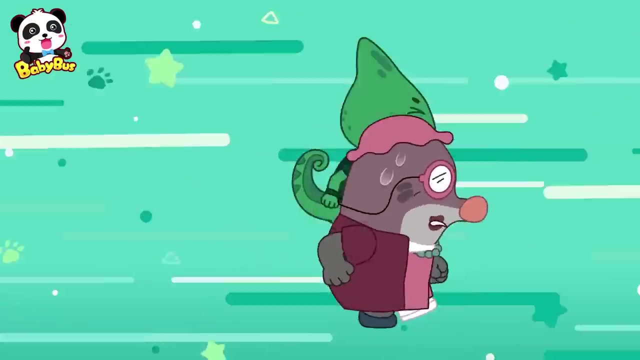 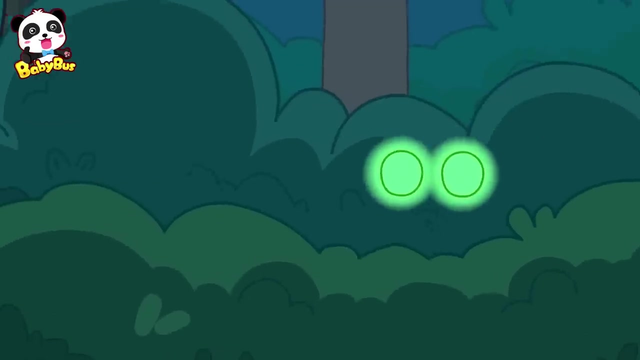 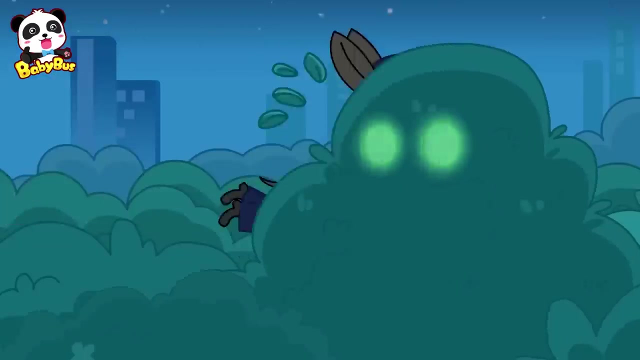 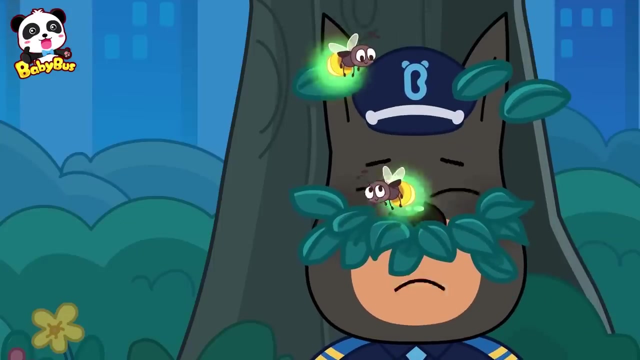 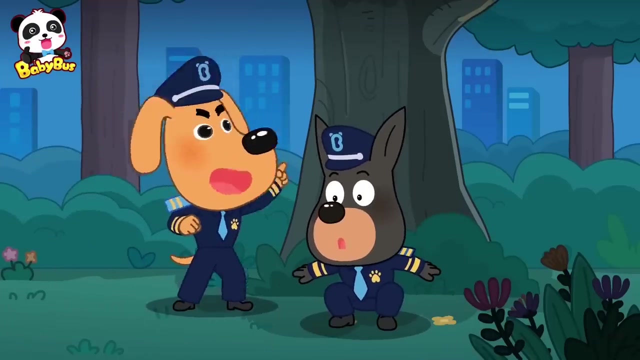 Coffee Go Run. The ghost is coming. Ha, Who's there? Yaaaaaah, Huh, Huh, Huh. They are fireflies. Huh, Huh, Oh Huh, There it is. 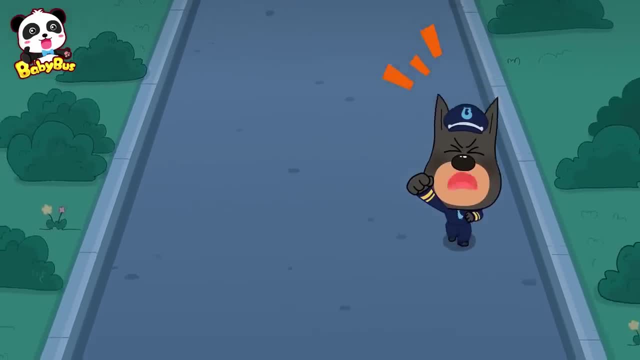 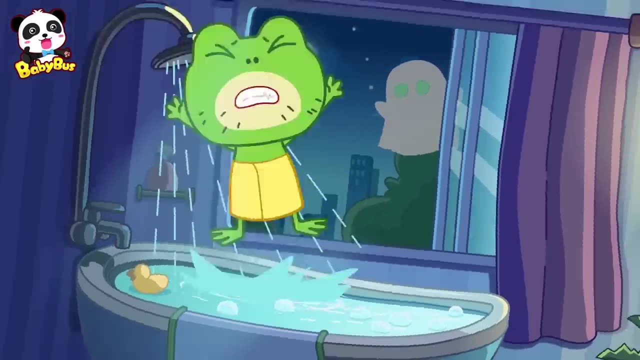 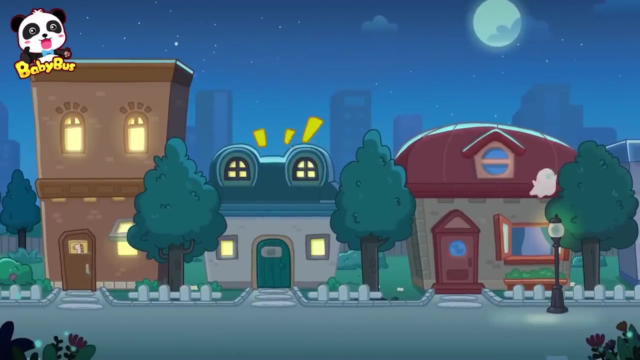 Stop right there, Ha, I'm gonna get you. Uh Huh, Aargh Ribbit It's-a ghost Ghost. It's-a ghost, Ghost, Ghost. It's-a ghost Ghost, It's-a ghost. 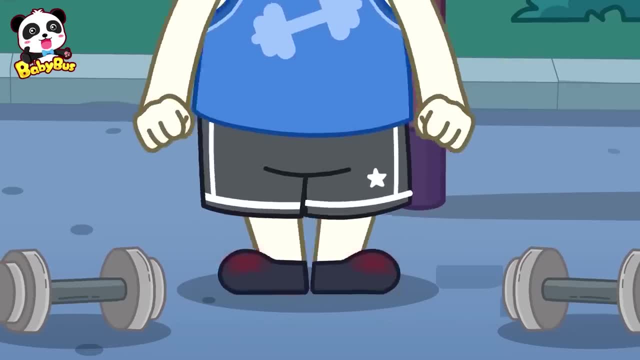 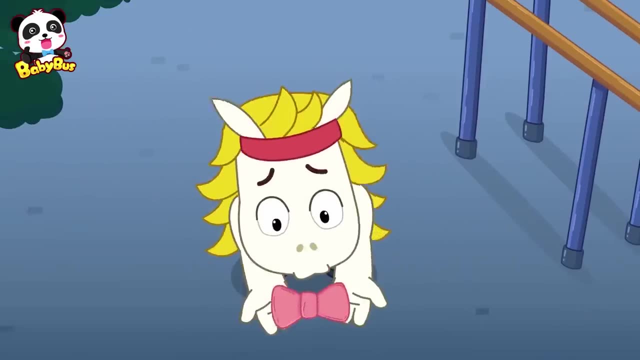 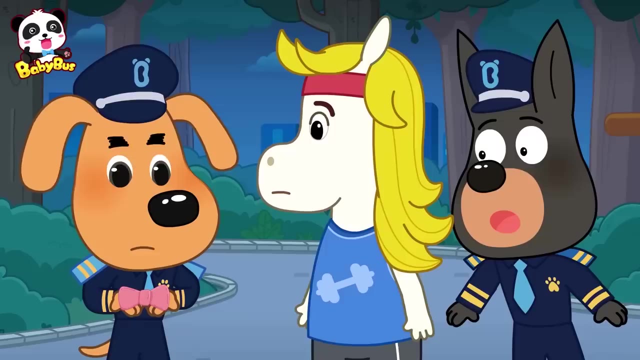 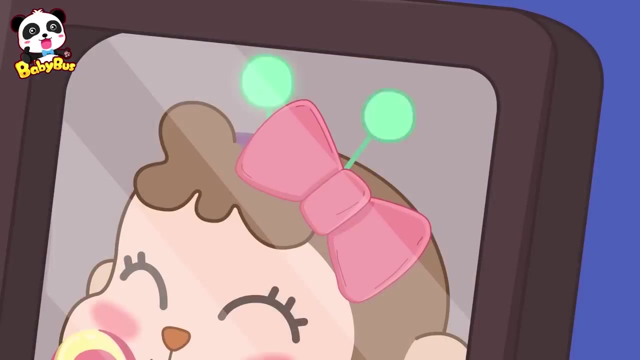 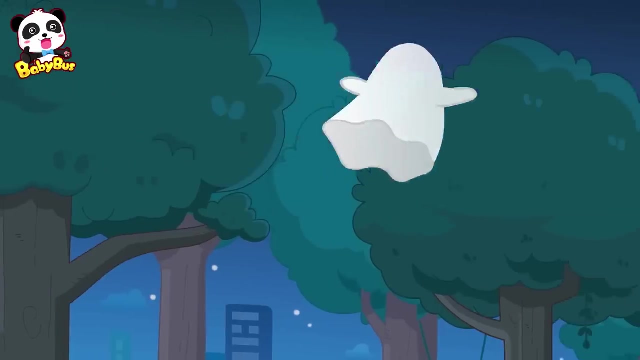 Ghost Gagh. Oh, Oh-ho-ho-ho, Huh, Ah, Ah. Sheriff Labrador, the ghost has distraught this: A ribbon And a flashing headband. I know what it is. No one can run away from me. 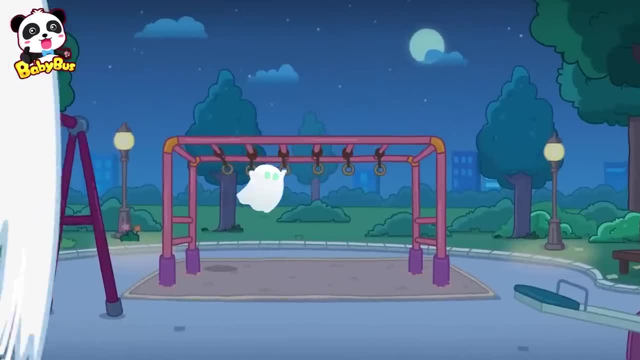 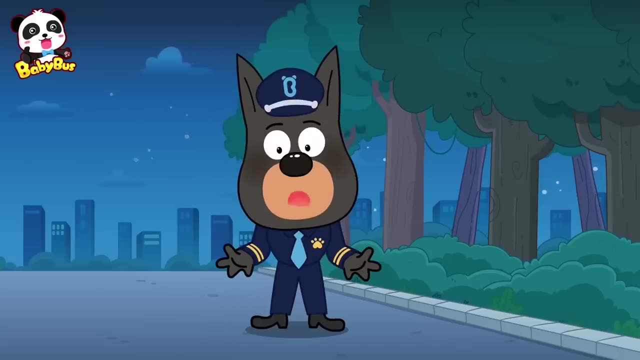 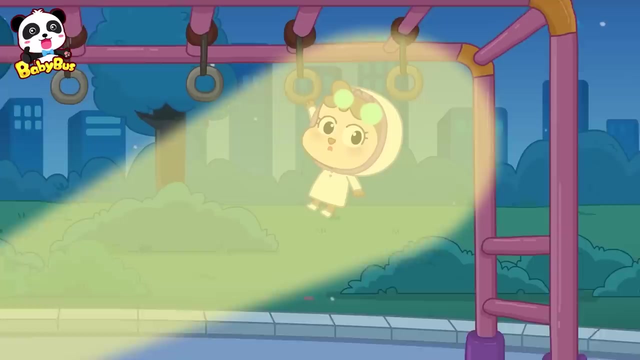 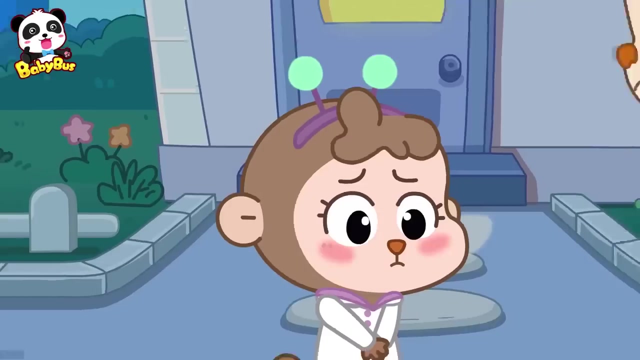 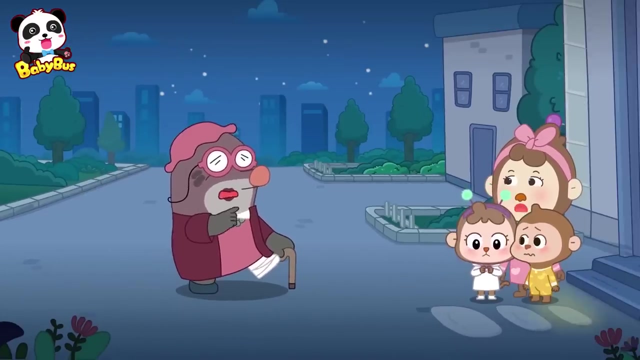 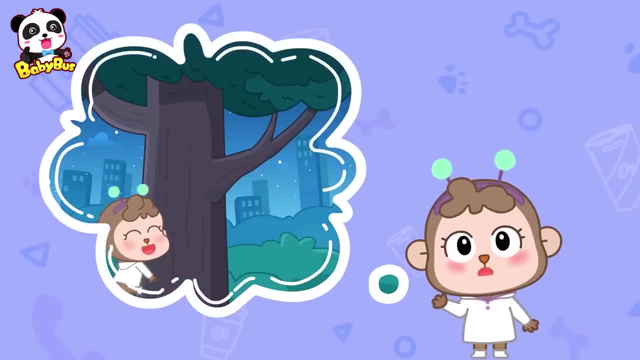 Why are you helping the ghost? It's not a ghost, It's Sister Monkey. So it was Sister Monkey, Sweetie. The children should be sleeping. Why are you scaring people like that? I'm sorry, I couldn't fall asleep so I came outside to play. 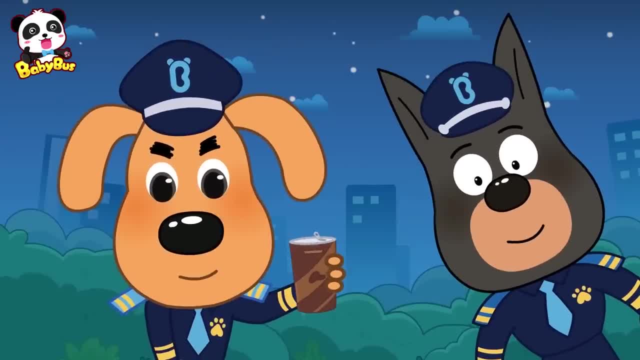 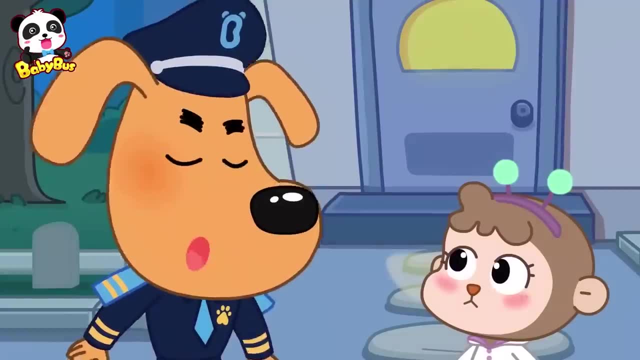 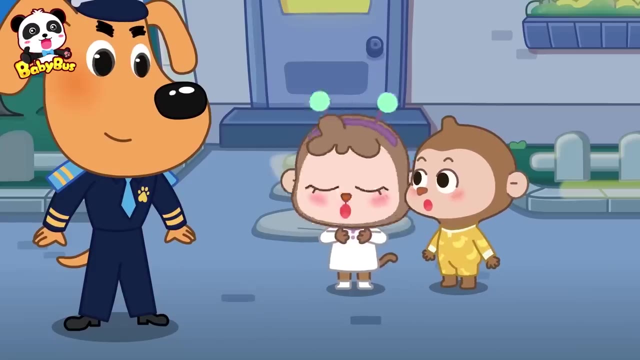 Sister Monkey, did you drink this? Yes, I was thirsty, so I took it from the fridge and drank it. Coffee is for grown-ups. Children can't sleep if they drink it. Oh, I see, I'll be careful of what I drink from now on. 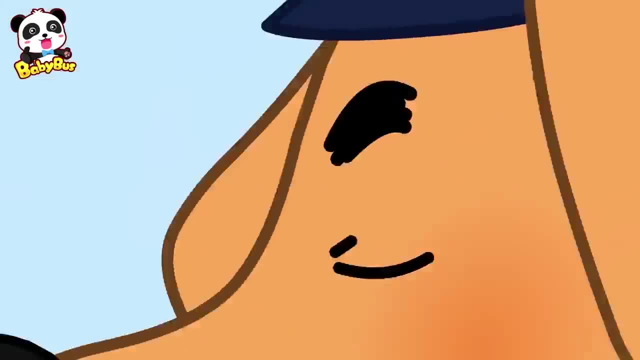 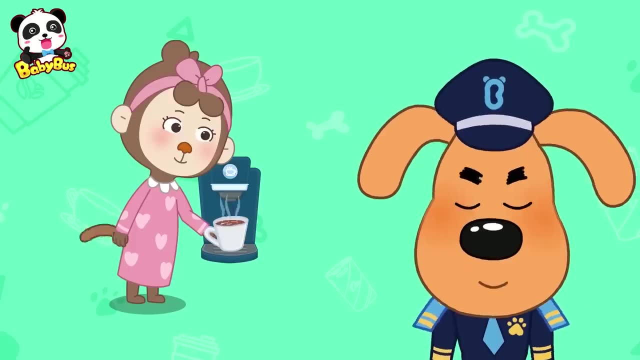 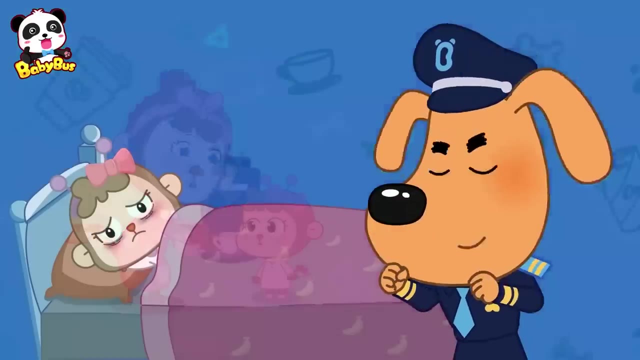 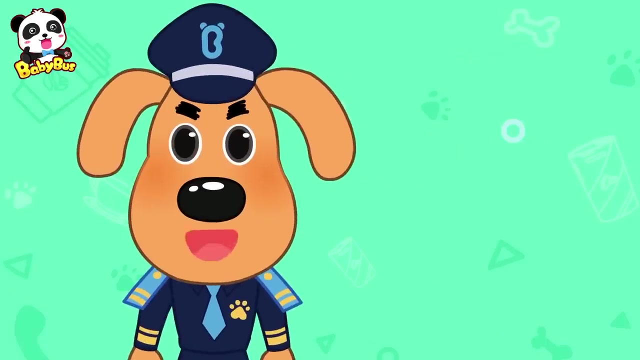 Okay, fine, Sheriff Labrador's Safety Talk. Kids coffee is a drink that's only for grown-ups, Because if children drink coffee, they can't fall asleep at night And it's not good for their health. Also, tea and drinks that contain alcohol are not for children either. 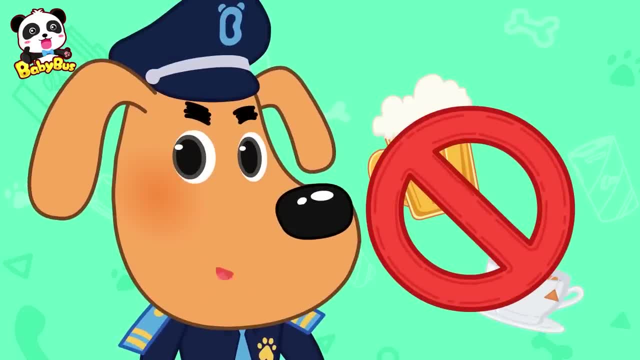 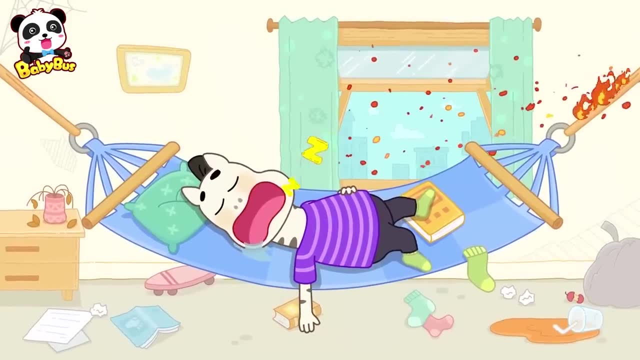 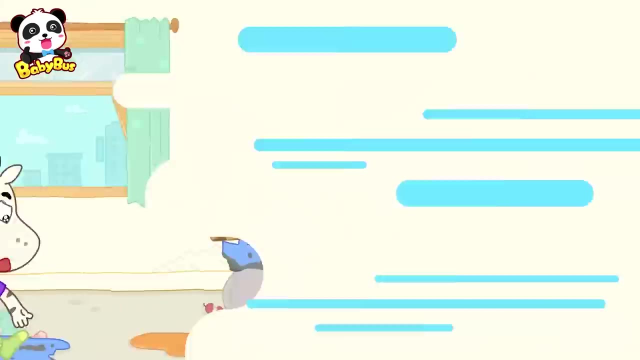 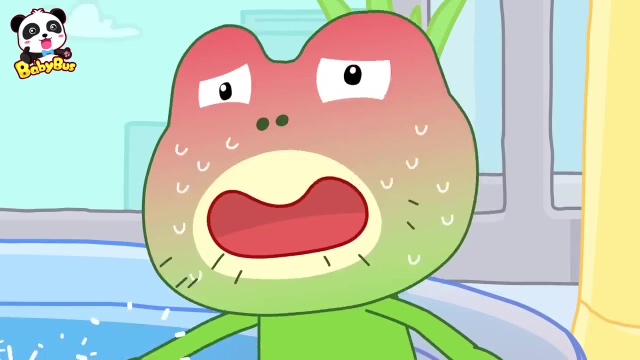 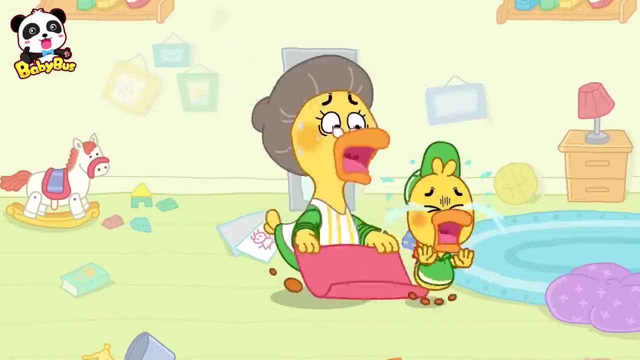 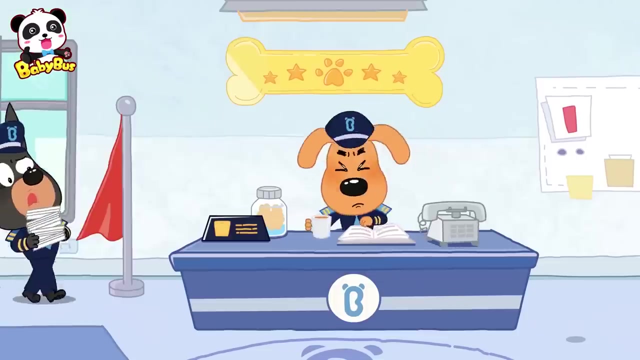 And you shouldn't drink them. Please keep that in mind. Woof. Fire at the duck's house. Oh, It's so hot. Help, Help, Quick, Quick, Quick, Quick, Help, Help, Help Woof. 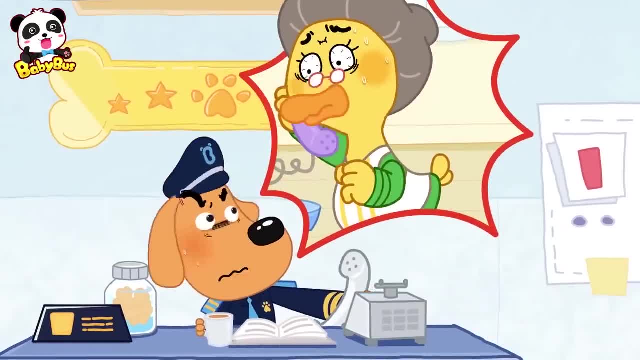 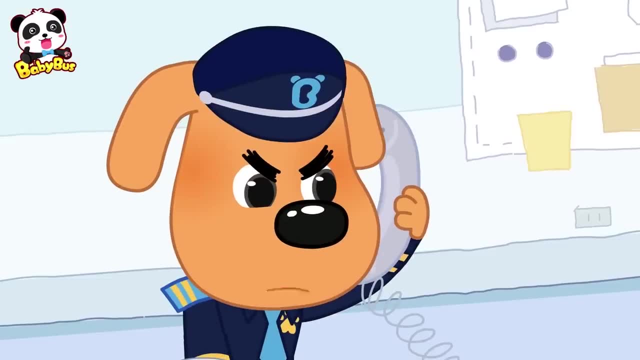 Hi, I'm Sheriff Labrador. Help, Sheriff Labrador. It's Granny Duck. We're on fire here. Quack, Quack, Quack, Quack. Don't worry, Granny Duck, I'll call the fire station first and we'll be right there. 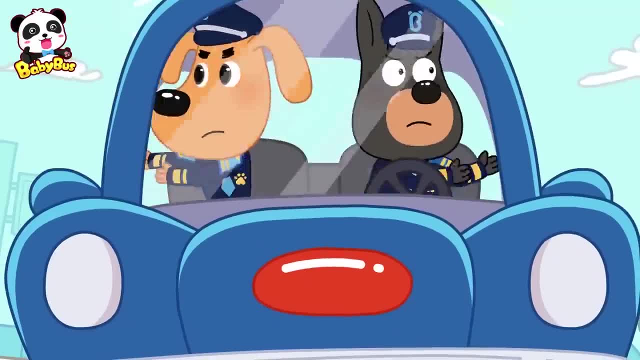 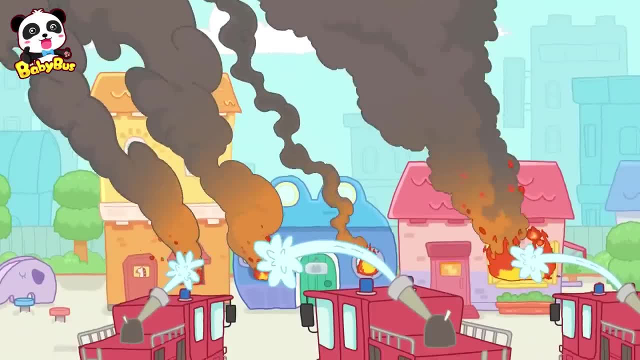 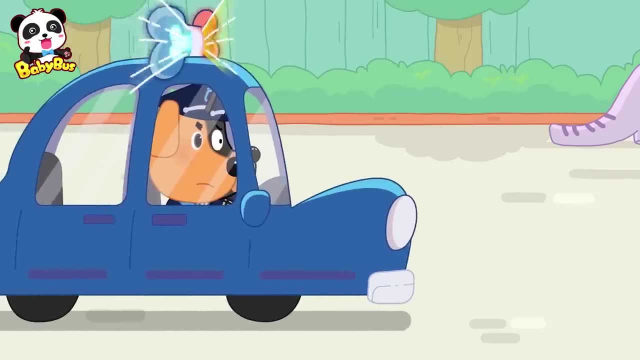 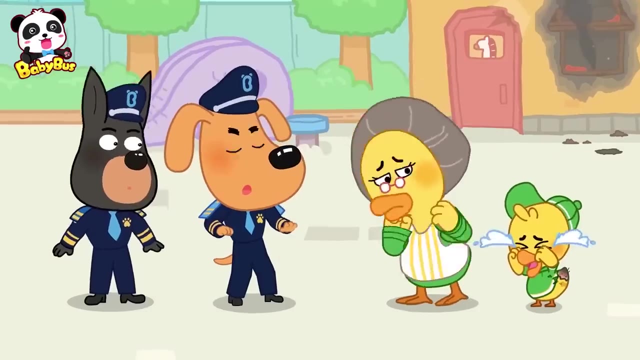 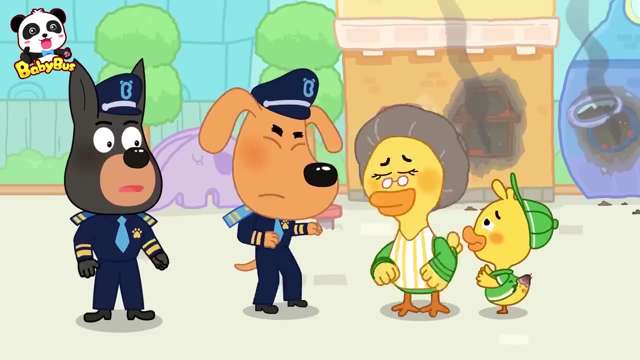 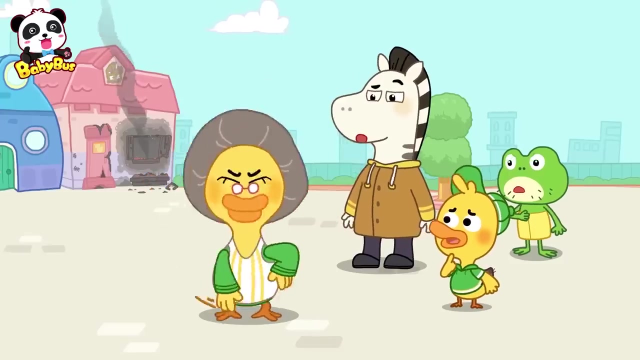 Quack, Quack, Quack, Quack. Sheriff Labrador, My poor little duck almost burned his tail off. Please help us. You must arrest the arsonist. Do you mean someone set this fire on purpose? Of course, Of course, Cher Labrador. You know what. 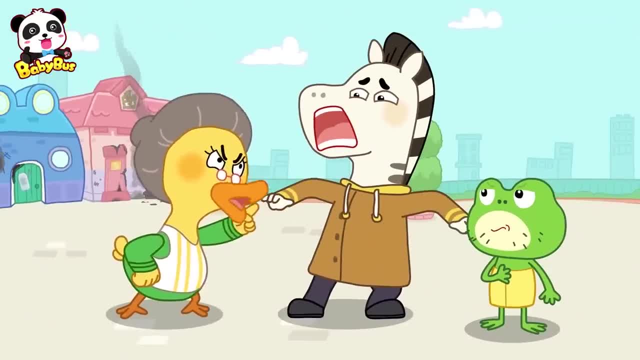 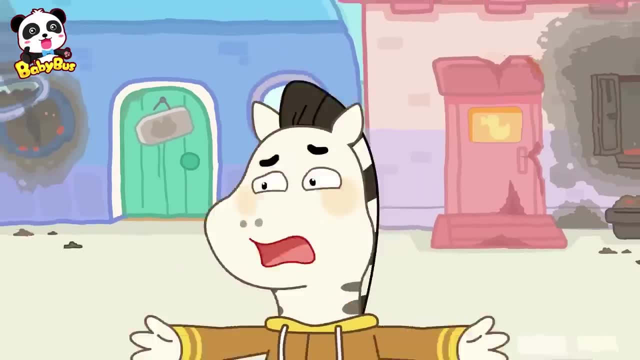 The last fire was started by Zebra as he dried his stinky socks on the stove Right. It must be Zebra again. I almost got roasted Ribbit. No, not me, I promise. I stopped doing that a long time ago. 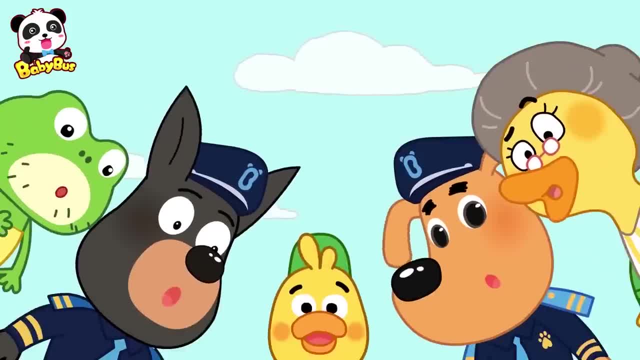 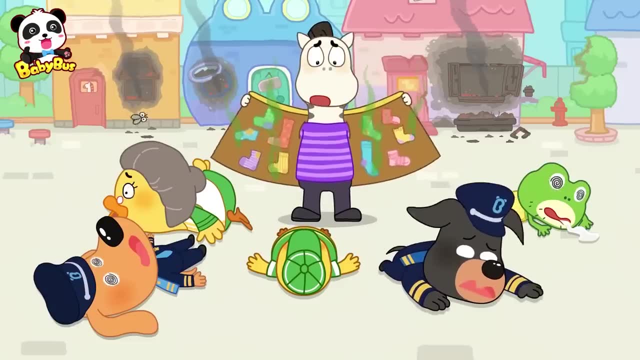 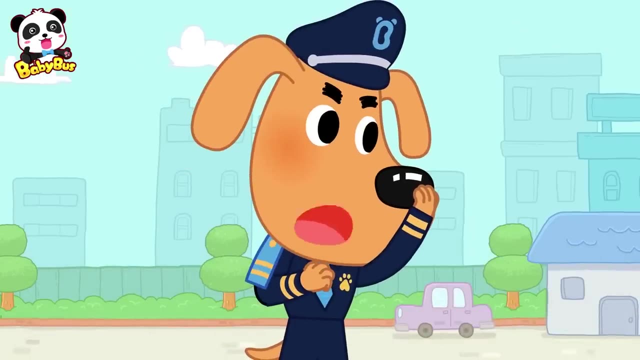 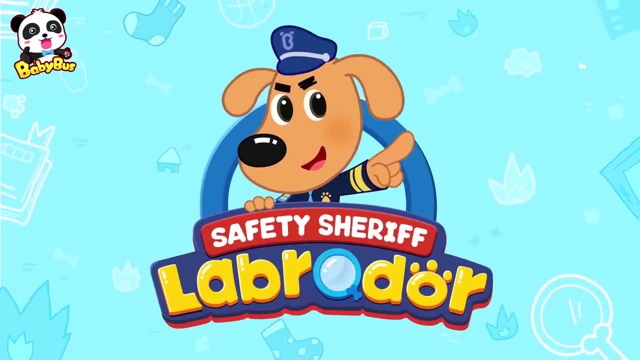 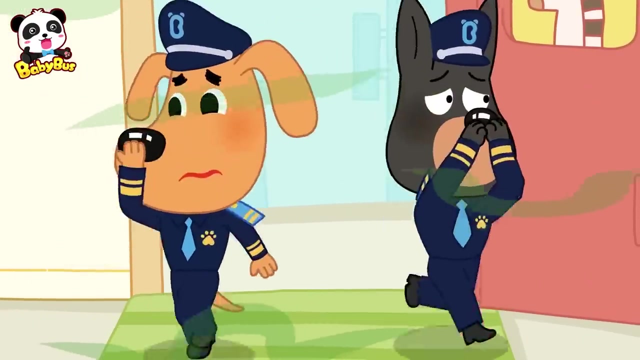 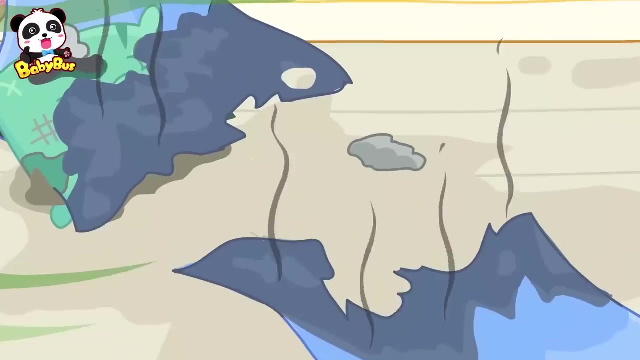 Look, you see, My socks are all right here. Don't worry, I'll find out the truth, Doby. let's go check Zebra's house Copy that It stinks. Only the hammock was burned. It's not the place where the fire started. 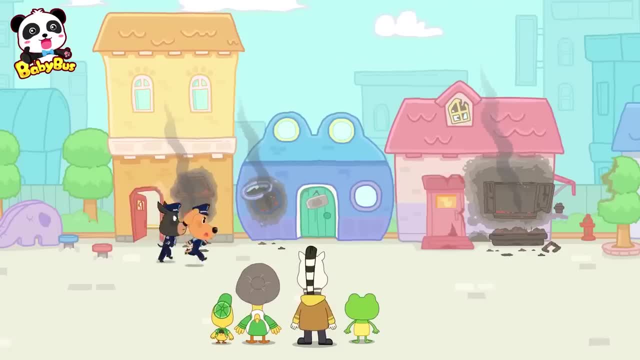 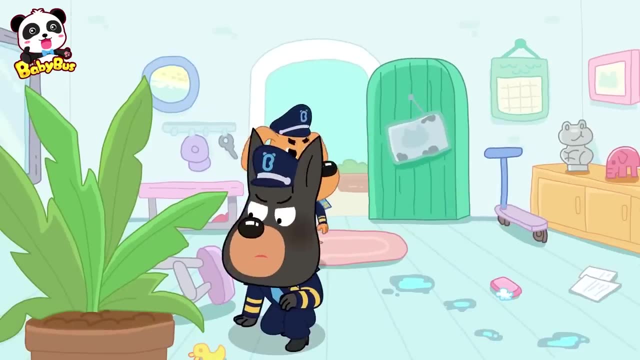 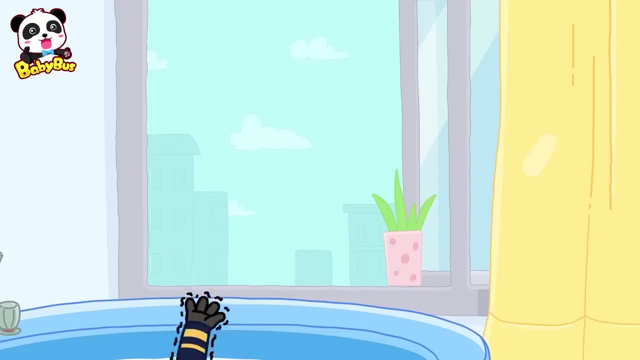 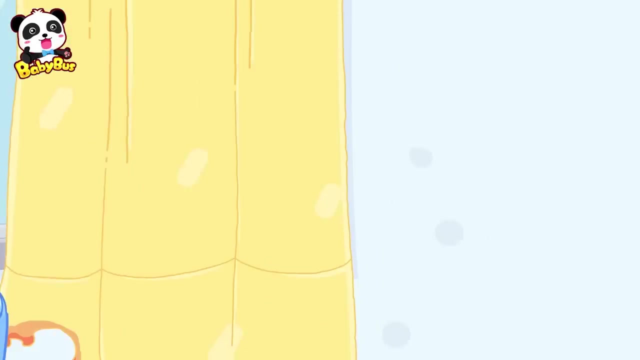 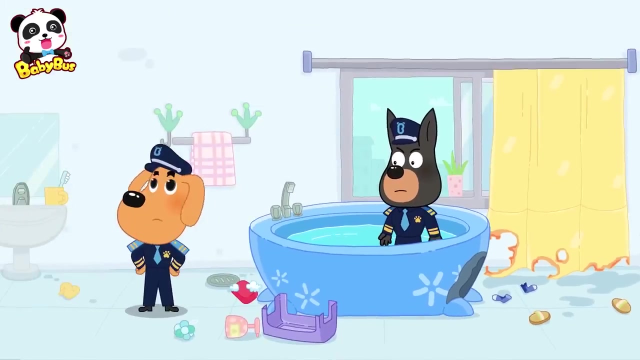 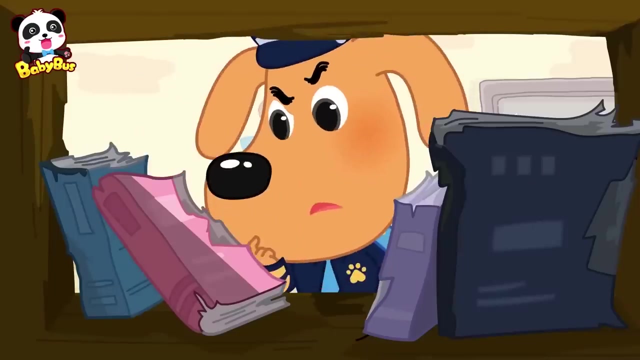 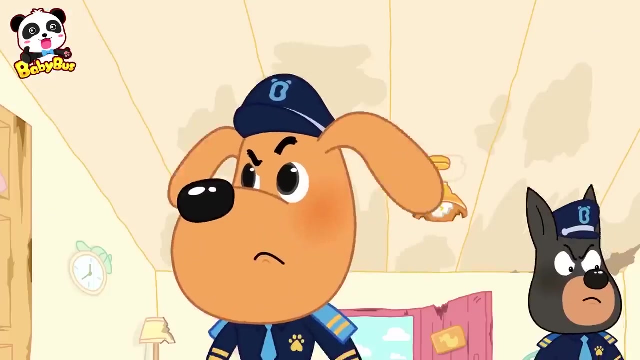 Let's go to Frog's house now. Sir, the only thing burned in Frog's house is the shower curtain. So it's not Zebra and not Frog. That leaves only the Ducks' house. Everything is burned here. This must be where the fire started. 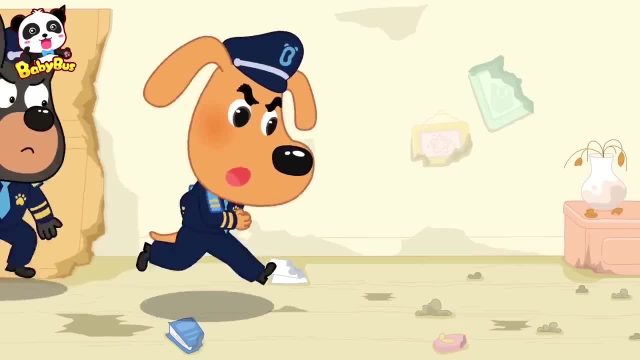 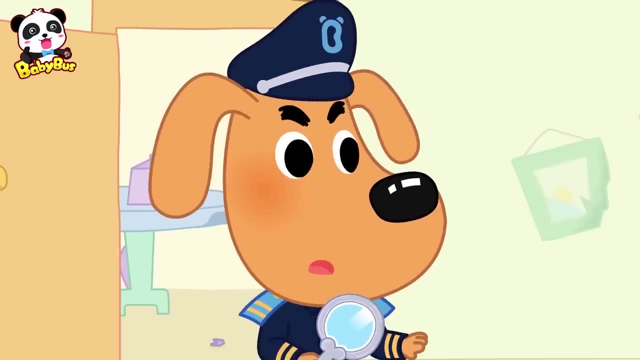 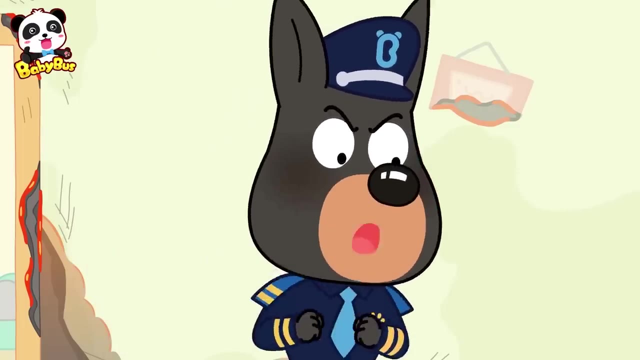 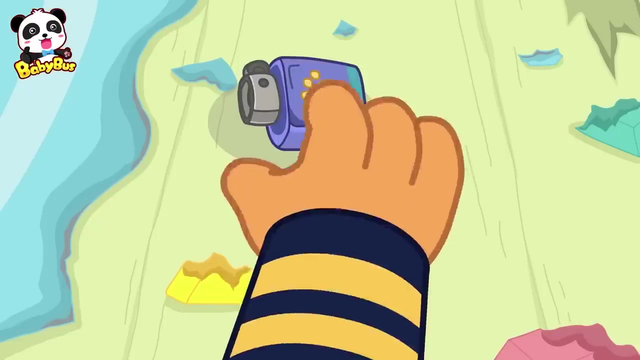 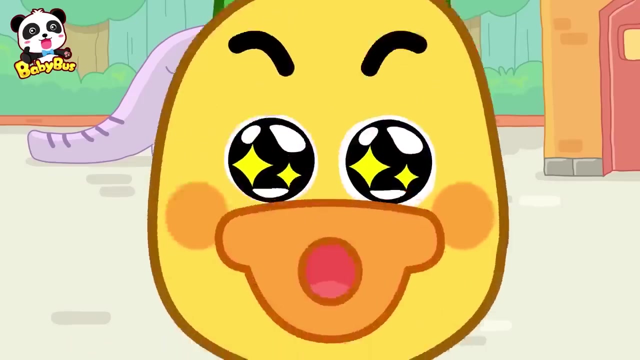 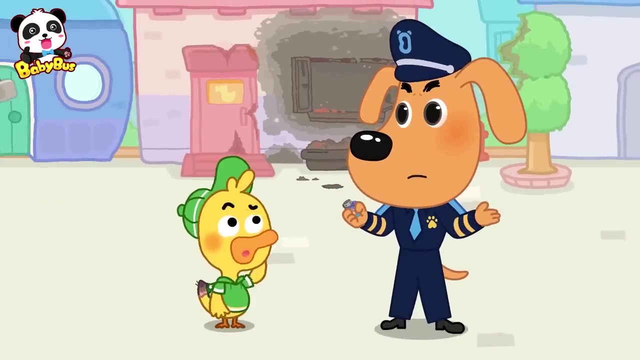 I think I smell the evidence. Huh, I think the answer is under the bed. Now it's my showtime. Huh A lighter. Hey, There it is My toy. Huh, The truth is, Little Duck is the one who caused the fire. 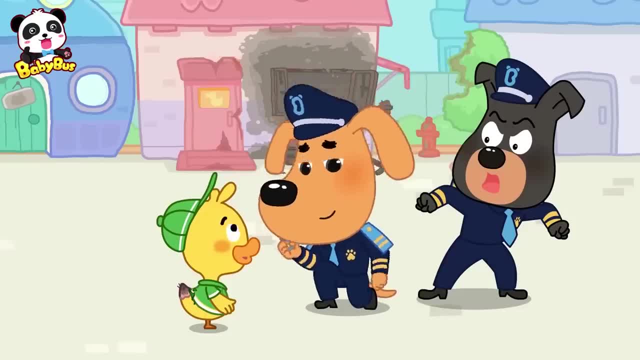 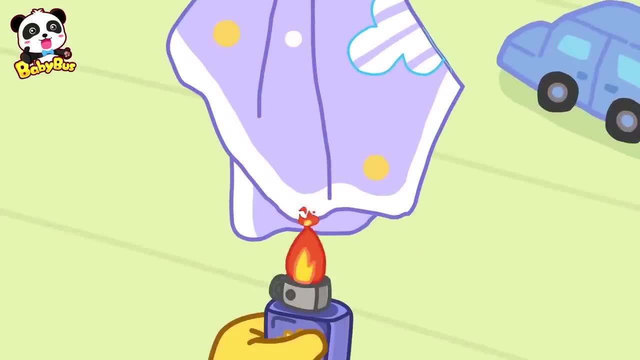 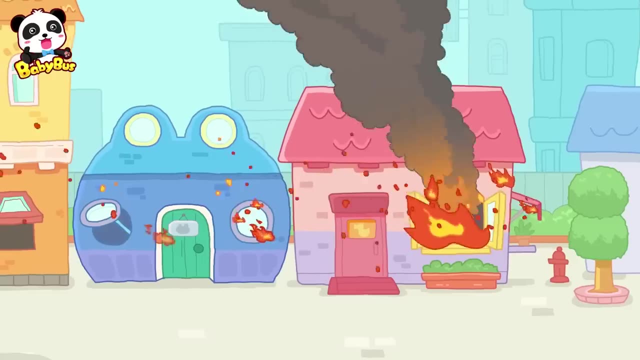 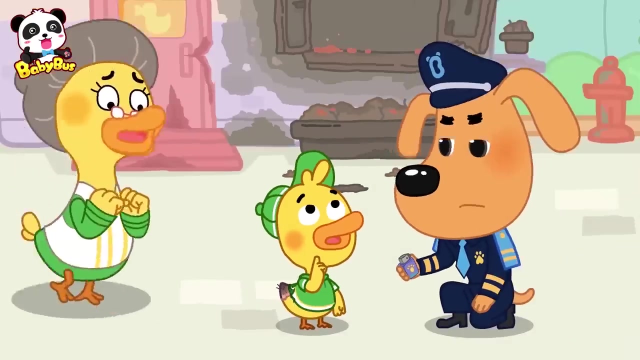 What? How can that be, Little Duck? what did you do with this lighter just now? Uh, just now it was like this: Huh, Oh, good heavens. So that's it. Oh my, I can't believe it.